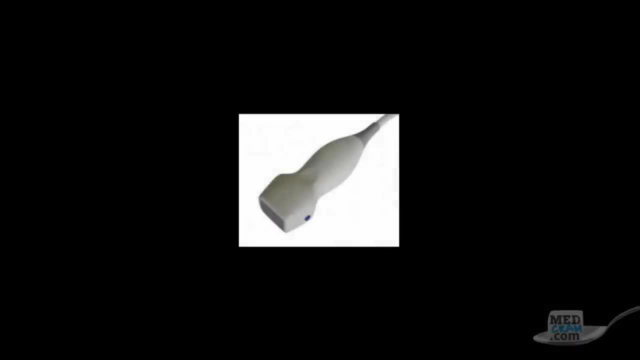 on the ultrasound screen And, if you notice, on every ultrasound transducer there's an indicator. That indicator may be a dot, as in this example, There may be a small protrusion, But nonetheless there's some sort of marking on the ultrasound probe and that is the transducer's indicator. 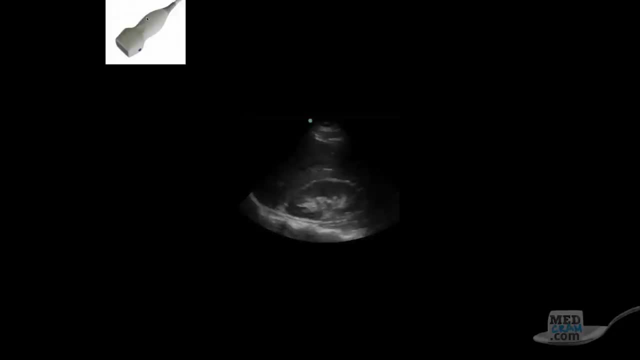 This corresponds with the indicator on the ultrasound screen, In this case a blue dot. It may be some letter or a proprietary symbol, but there'll be some indicator on the ultrasound screen that corresponds with the indicator on the ultrasound probe. You'll notice that. 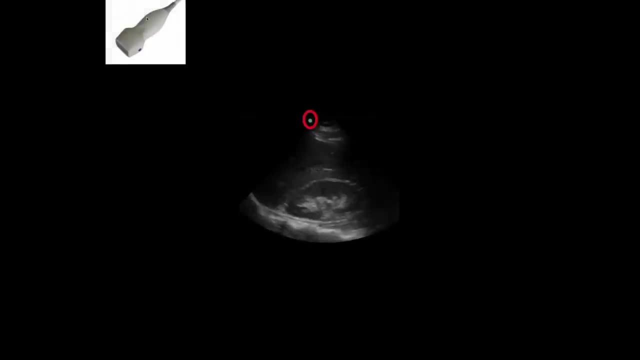 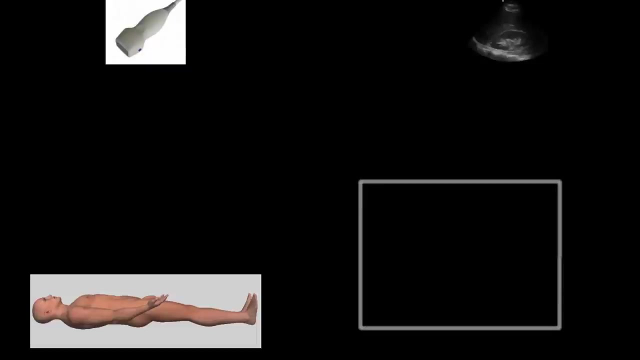 this indicator is the indicator on the ultrasound screen. You'll notice that this indicator is on the left side of the ultrasound screen. So how does this work? Well, we have our patient on the left and our ultrasound screen here on the right. We're going to place 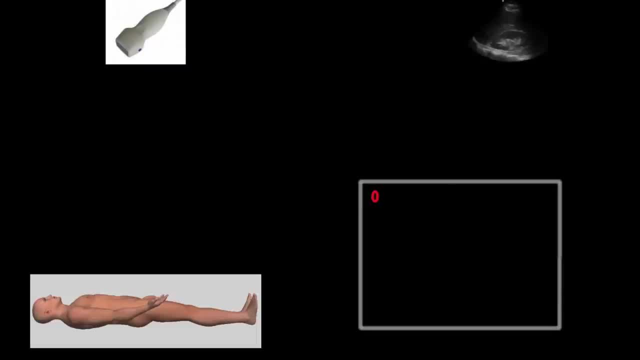 the ultrasound screen indicator on the left side of the screen. So if I place my ultrasound transducer on the patient and I point the indicator towards the patient's head or superiorly, that lets me know that where the indicator is on the screen, in this case the left side. 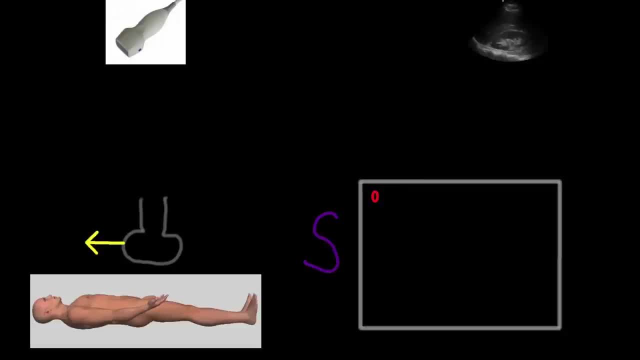 then is the ultrasound screen And apparently the goin' counselor or the Auditory is an individual or the himself that is gonna be working outside. You might not want to point, because the later loss is easier to answer. Okay of the screen correspond to. So now let's look at what the top and the bottom of the screen 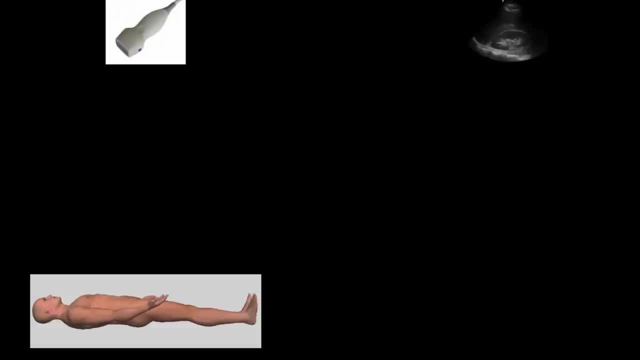 correspond to, And to do that we have to think of our ultrasound probe as a flashlight. So if I place my ultrasound probe or my quote-unquote flashlight on the patient, where is the ultrasound beam shining from and where is the ultrasound beam shining to? Well, in this case, the ultrasound. 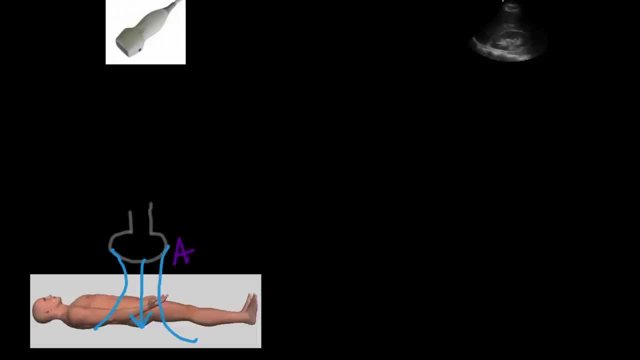 beam is shining from the anterior of the patient toward the posterior of the patient. So then, on my ultrasound screen, the near field or the top part of the screen is anterior and the bottom part of the screen is posterior, because that is where I'm shining my beam from and where 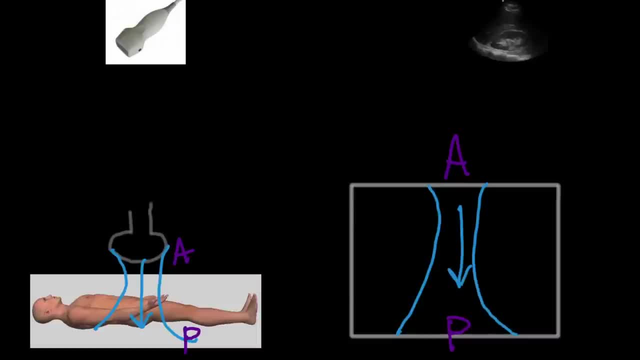 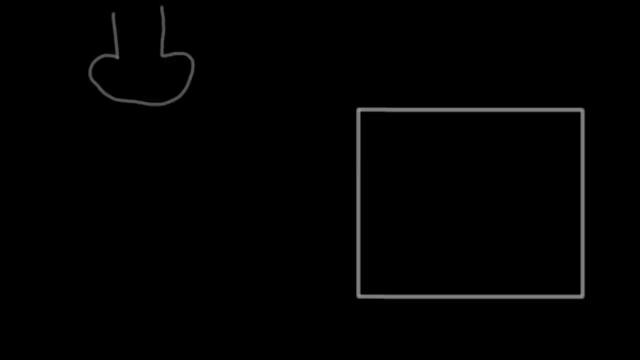 I'm shining my beam to. So we're going to do some examples that will more solidify the picture, This concept. Well, you'll notice that we asked ourselves two questions And if we ask ourselves these two questions, we can always find out the orientation of the ultrasound screen And the 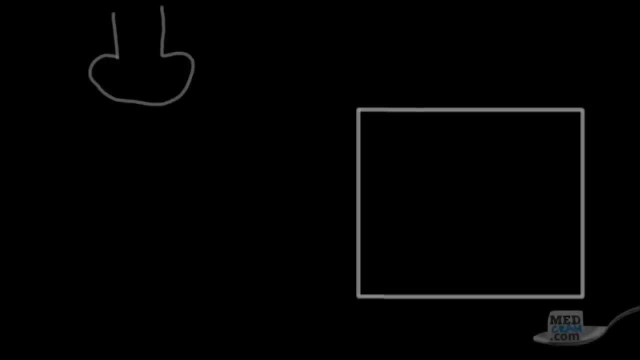 first question is: on my ultrasound transducer, where is the indicator pointing? And that is going to correspond with where the indicator is on the screen, And then the opposite of that will be true. So if the indicator is pointing on my ultrasound transducer, where is the indicator pointing? 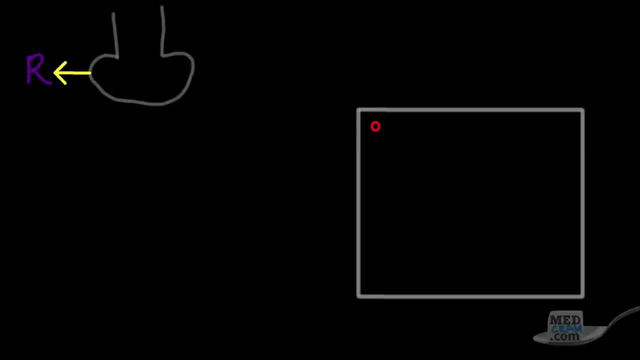 Towards the patient's right, then the left side of the screen, since that's where the indicator is, will be the patient's right. The opposite of the indicator, then, would be the patient's left, And that figures out what's on the left and right of the screen. The second question we need to ask: 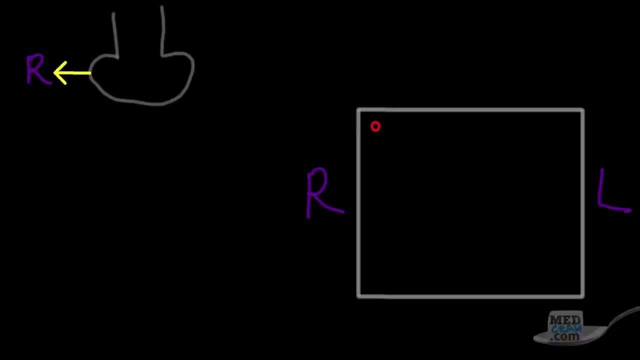 ourselves then is: where is the ultrasound probe shining from and where is it shining to on our patient? If it's shining from the patient's anterior body to the patient's posterior body, then that will correspond with the top of the screen being anterior and the bottom of the screen 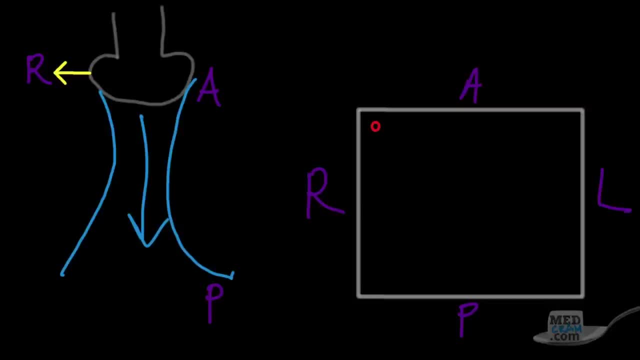 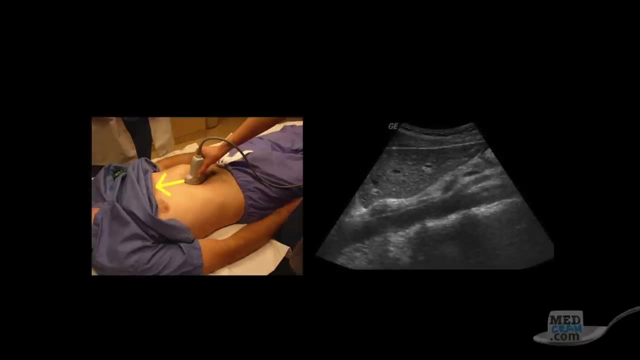 being posterior. So now let's do some examples. The first example: here we have our patient on the left and we see that our indicator is pointing up towards the patient's head or superiorely. So that means that the left side of this screen 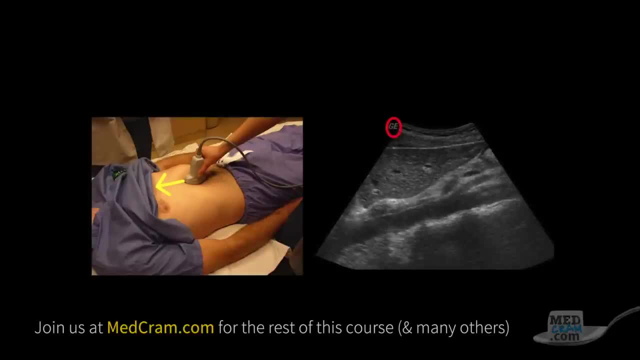 because we have the indicator here on the left side, is going to be superior and the opposite of that then is inferior. And we see on this patient that our flashlight is shining from the anterior portion of the patient to the posterior portion of the patient. Therefore, the top of the screen is anterior, the bottom of the screen is posterior. 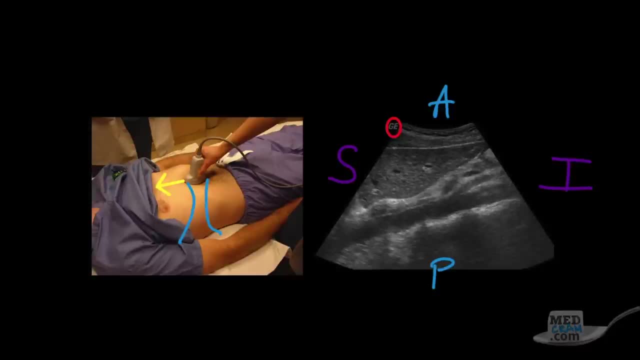 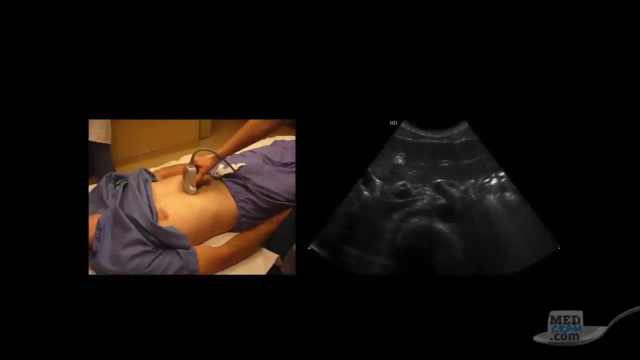 If we put this in conventional anatomic planes, this is the sagittal plane And this is because we're slicing the patient with the ultrasound beam in a sagittal plane. Okay, next example: We see on our patient on the left here that our indicator is pointing towards the patient's right. 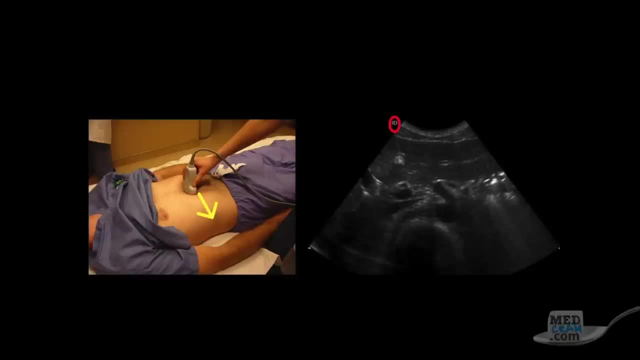 and our indicator on our screen is on the left side of the screen. That lets us know that the patient's right is on the left side of the screen and the opposite, then the patient's left is on the right side of the screen. 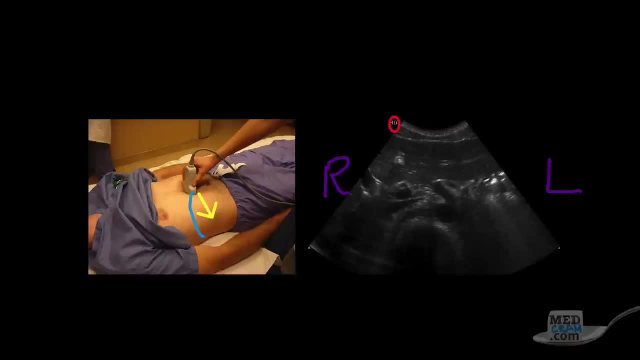 And then we see that our ultrasound beam is shining from anterior to posterior again. So the top of the screen is anterior, the bottom of the screen is posterior And therefore this is your classic transverse or axial plane. And this is just like an axial or transverse slice on a CAT scan or MRI. 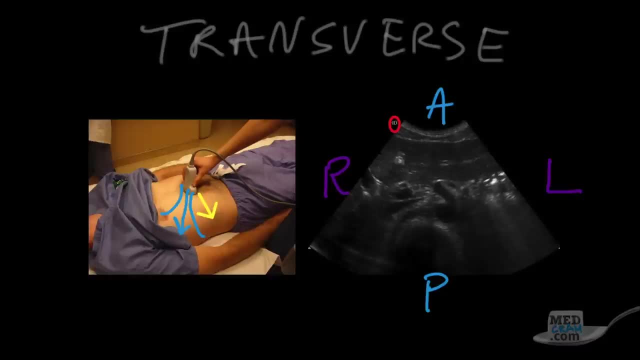 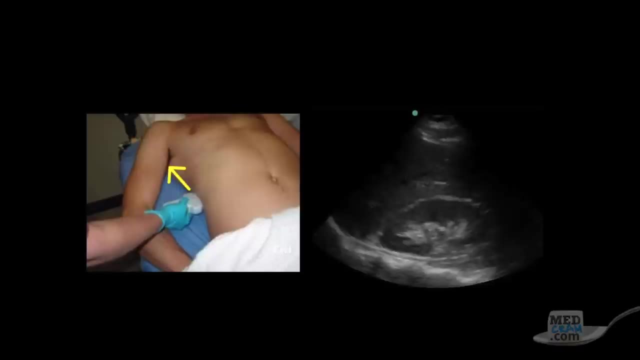 where you're looking at the patient from the feet towards the head and then you're looking at the patient from the side of the screen and then you're looking at the patient from the side of the screen. Next example: we see that our indicator is pointing up superiorly on the patient and that our indicator on the ultrasound screen is on the left. 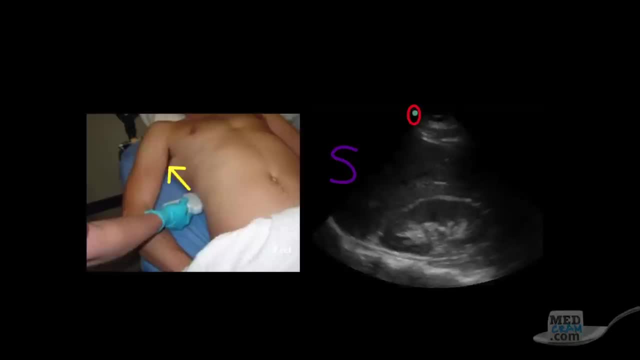 Therefore, the left side, again, is superior, and the opposite of that, then, is true where the right side is inferior, And in this case, our ultrasound beam is shining from the right side of the patient toward the midline and then to the left of the patient. 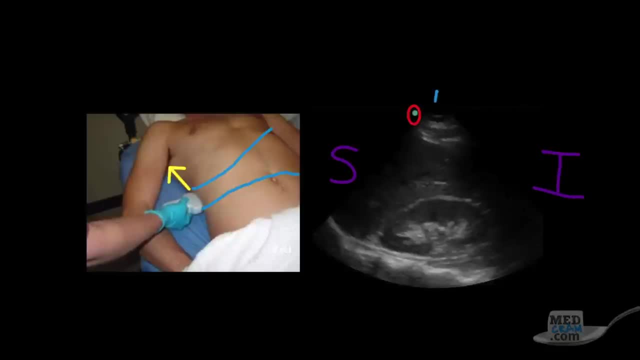 Therefore, the near field, or the top of the screen, is going to be the patient's right and the far field is going to be the patient's left, And this is a classic coronal slice from the patient's right to the patient's left. 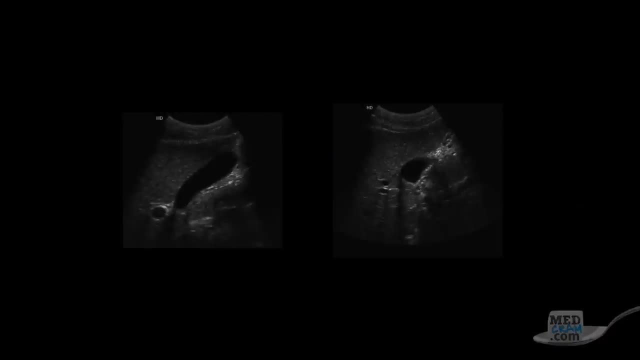 Now we looked at the three classic imaging planes. but sometimes structures do not lie in those classic planes. An example is the gallbladder. Here we see the outline of the gallbladder, And the gallbladder does not sit in the same plane on every single person. 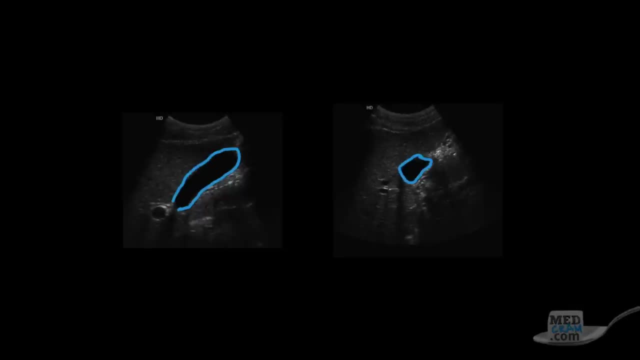 So instead of imaging in planes, we're going to image in long and short axis in relation to the structure. So this would be the long axis of the gallbladder and this would be an orthogonal plane or 90 degrees from that long axis.